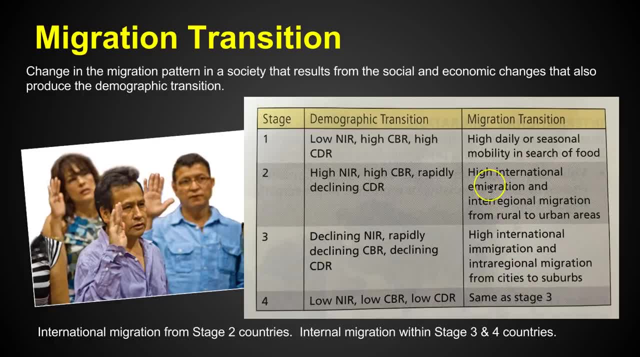 cities to the suburbs. In stage two, we're seeing international migration from the cities to the suburbs, migration where people are moving from the country to cities. In stage three, we're seeing them go from the cities to a better lifestyle in the suburbs. Within stage four, we remember that the birth rate is low. 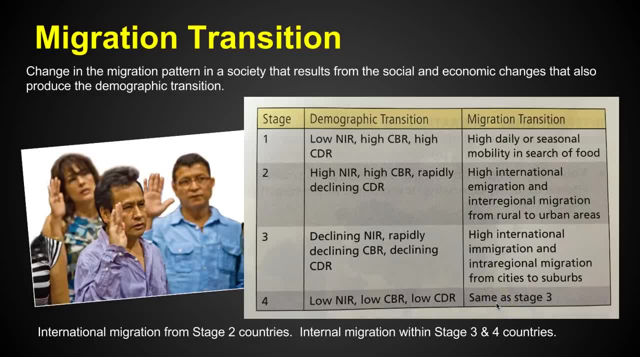 and the death rate is low. So the situation is going to be the same as in stage three. People are still going to be traveling internationally in search of jobs and a better life, but within the country, they're going to be leaving the cities to go to a better lifestyle in the suburbs. In stage two, 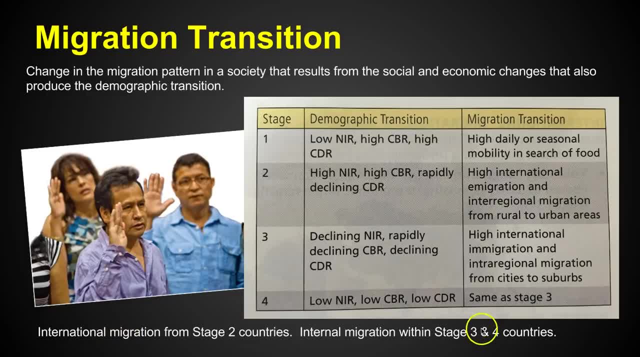 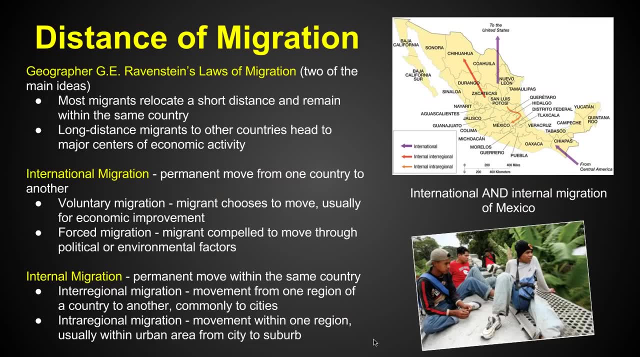 we see international migration. This is the most prevalent In stage three and four. we see internal migration, where we're going from the cities to the suburbs. Distance of migration. Geographer GE Ravenstein created laws of migration and two of the main ideas that you need to understand for AP. 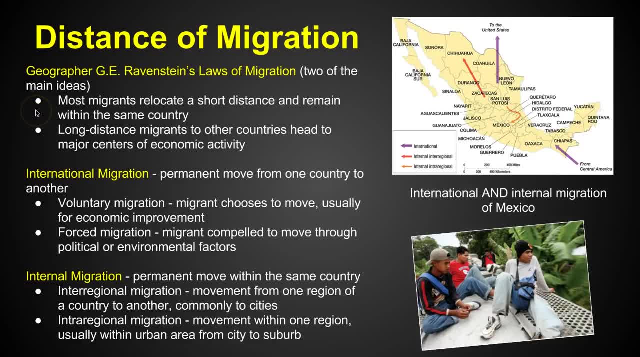 human geography were that most migrants relocate a short distance and remain within the same country. The second principle was that long-distance migrants, they move to other countries, head to major centers of economic activity, usually cities. So most migrants they stay within the same country and move around to find jobs. Most other migrants when they travel long. 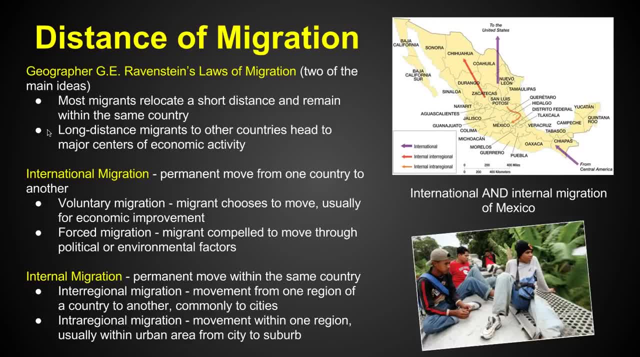 distances. they head to cities where they can find jobs and be with other people that are like them. There's two forms of migration: International migration, where it's a permanent move from one country to another, and internal migration within the same country, So within international. 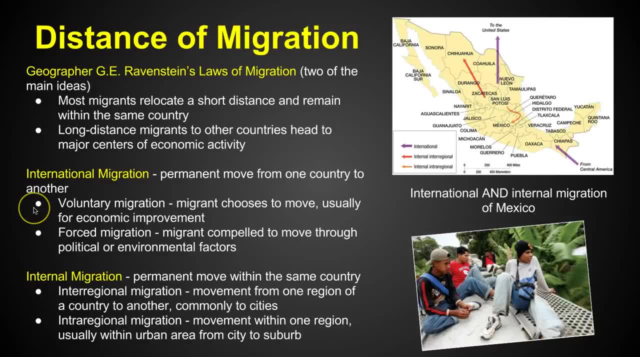 migration, where you're moving permanently to another country. there's two forms of that. We've got voluntary migration, where the migrant chooses to move, and they're usually moving for economic improvement, They're going to find a better job or a job. And there's also forced migration, where 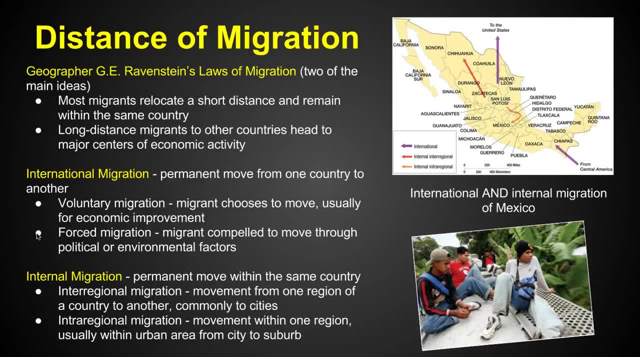 the migrant is compelled to move through political or environmental factors, like something is causing them to move. They don't really have a choice: Internal migration, migration within the same country permanently. You've got interregional migration, where you're moving to another country. 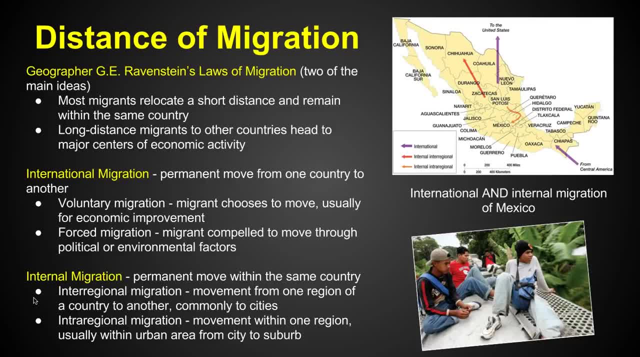 and people are just moving around the locally. So you select a region of the country where you're going to move to and there's movement within the other region. So typically you would see most of the lagrange more in the regional line of movement and komplett migration. 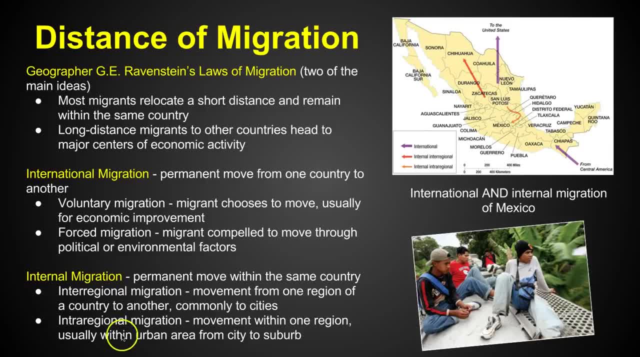 which is movement from one region of the country to another. So commonly we're seeing people move from the regions of the country to the region of the cities. And then there's also intra regional migration, where it's movement within one region, where we see 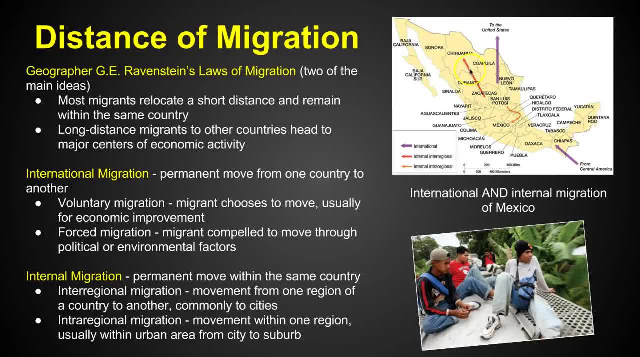 everybody's in, like a large city area, but really they're just moving within that region where they're going from the city to the suburbs and so they're going to maybe the poor area, to Chihuahua here, which is along the US border, where they're gonna have lots of work because factories from the 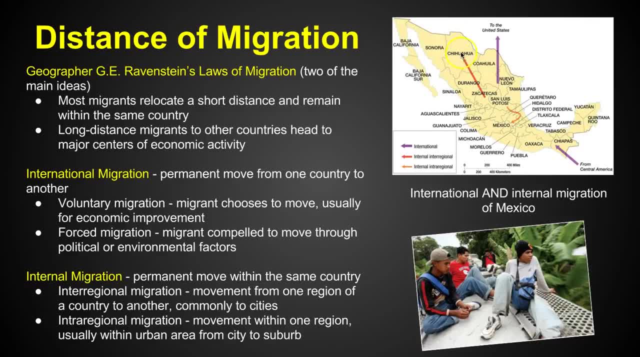 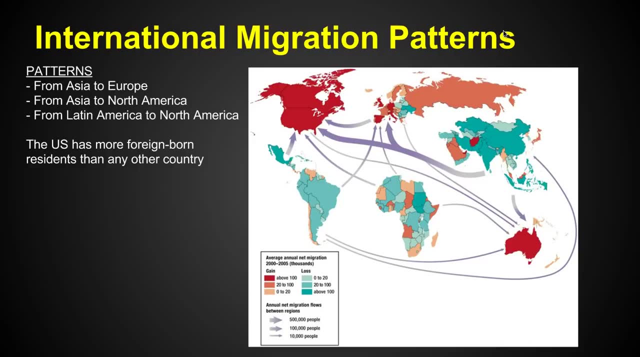 US like to set up right here, and so people will move to Chihuahua district to get jobs, but they will also do international migration, will then move from Mexico to the United States for jobs. international migration patterns. how are people moving across the earth? well, the patterns that we see, the ones 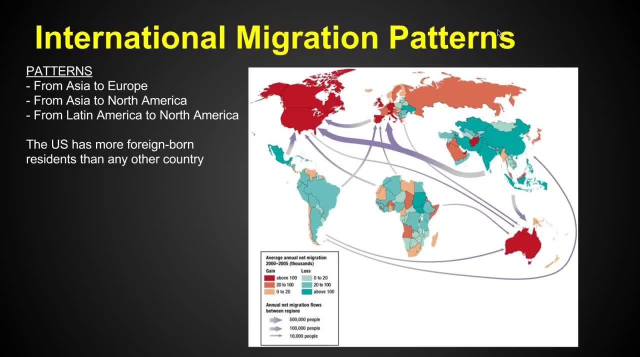 that are the most prevalent are people moving from Asia to Europe. so this is separated here so you can get the idea. but here's Asia and what we're seeing is people moved to Europe in search of jobs in a better lifestyle. the other pattern is from Asia to North America, again looking for a better 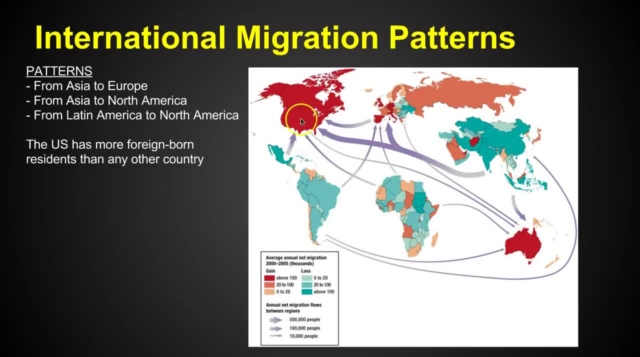 lifestyle, looking to get away from persecution and looking for jobs in United States. and the last pattern, that is the most common, is moving from latin america to north america. when you consider the top three patterns, these are it: asia to europe, asia to north america and latin america to north america. the interesting fact is that the united states has more foreign-born. 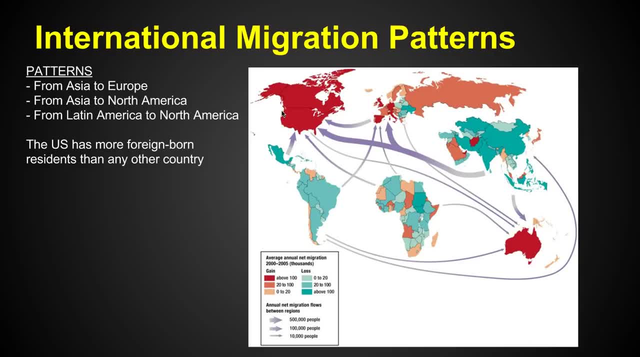 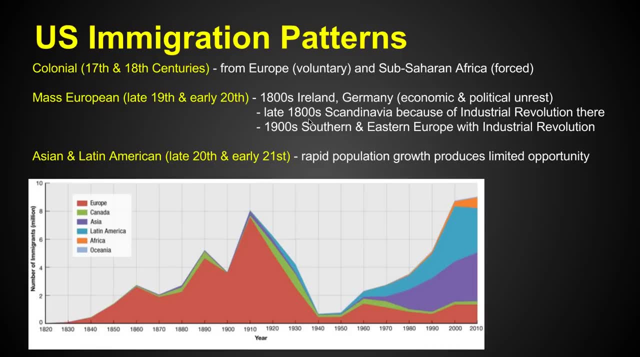 residents than any other country. so if you want to talk about the number one migration pattern, it's moving to the united states. us immigration patterns. what have we seen over time in this country? well, we have three different periods and you can see those periods spiked out here along. 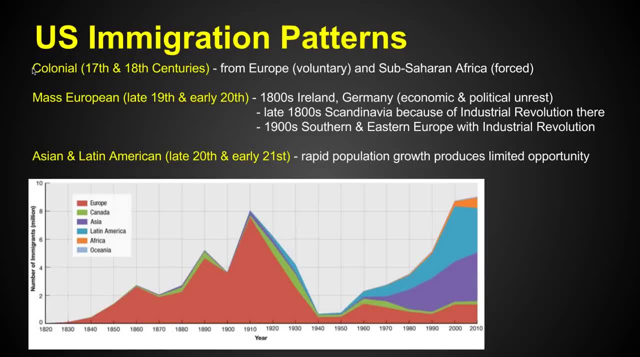 this graph. but the first period we look at is the colonial period during the 17th and 18th centuries. we know about this from middle school, studying it from history. these are when people come from europe in a voluntary manner to relocate, to start new lives in the new world. but we also see people 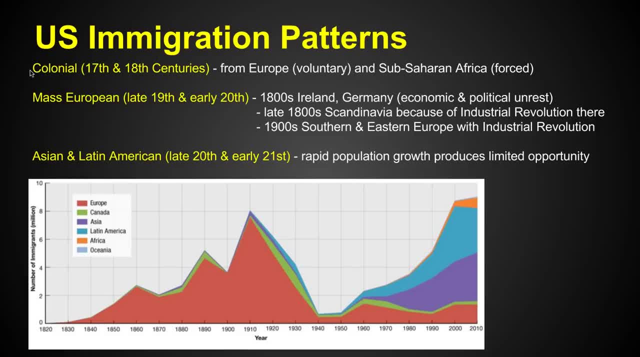 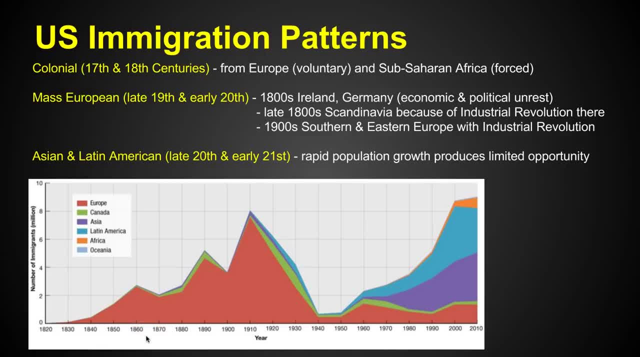 this is when we're seeing a huge spike. so the 17th century one is that that's the 1600s. the 18th century one is that 1700s. okay, so we're not even to that point yet. the second stage: we 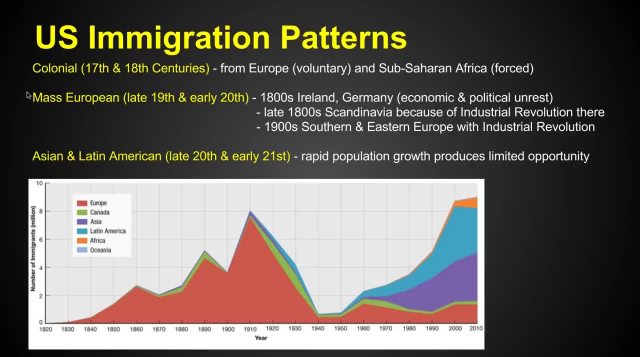 see is mass european migration during the late 19th and 20th centuries. the situation we have going on there in the 1800s in ireland and germany is there is enormous economic and political unrest. and you think about in the 1850s for middle school you should know all about the potato. 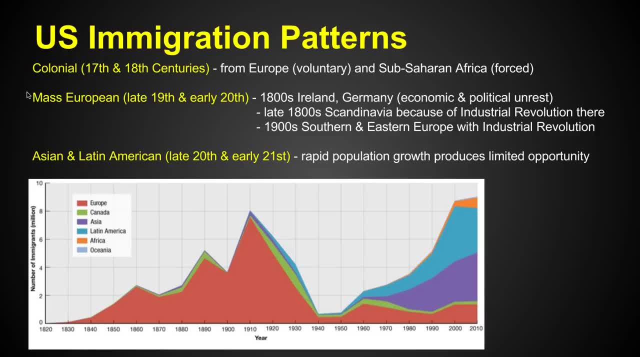 famine in ireland, which was the cause of huge economic downturn, and so people started to leave the country, coming to the united states. something else in the european area during the 19th and 20th centuries was that in the late 1800s people from scandinavia began to come over because the 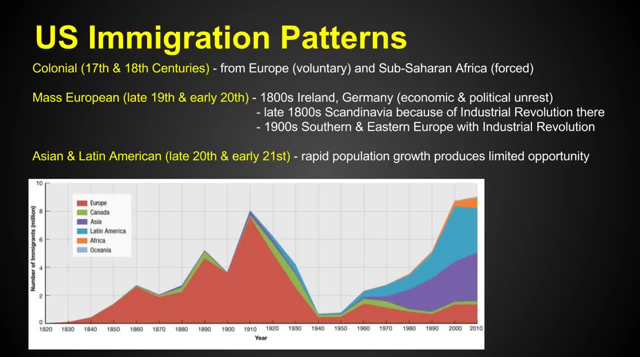 industrial revolution diffused to scandinavia. scandinavia is in northern europe and even northern east and eastern europe, so when you have the diffusion of the industrial revolution it creates mass population explosions and overcrowding. so people leave scandinavia as it diffused there in search of 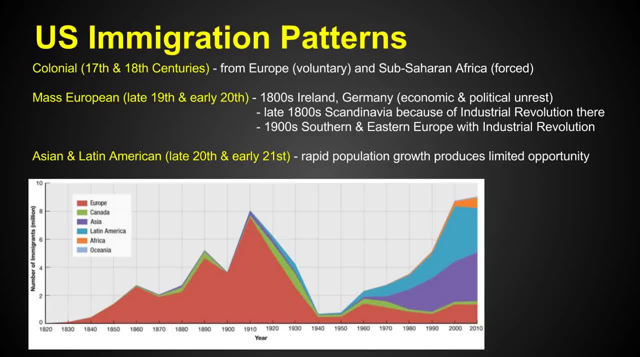 jobs in the united states and in the 1900s- the early part of the 1900s, we see people from southern and eastern europe started to come to the united states because the industrial revolution diffused there, and the thing about it is that the industrial revolution did create lots of opportunity and jobs. 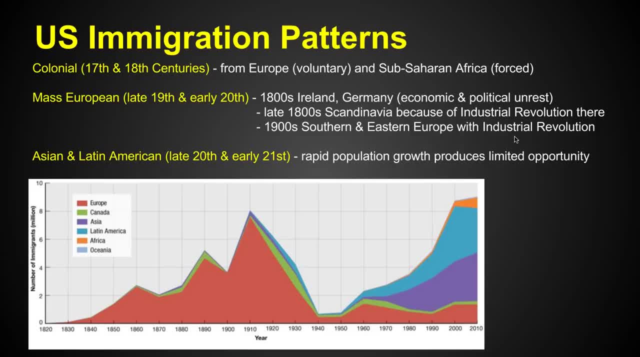 but along with that it created overpopulation, pollution, overcrowding, because everybody would move to those areas where they got the industrial revolution because they were looking for jobs. but it became so overwhelming that people were overcrowded, they were pushed out and they were pulled to the opportunity and land in places like north america. and this is what you saw during the 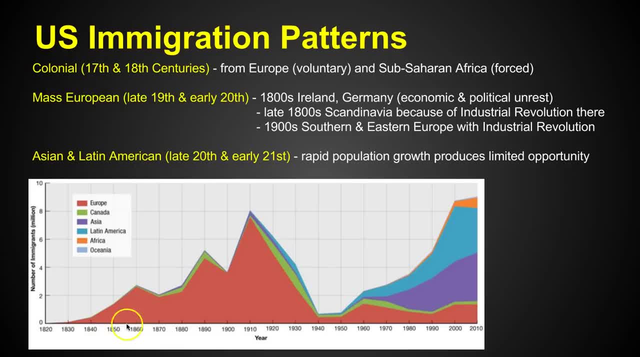 late 1800s and 1900s, which is where we see the spike right here. you know you think about the potato famine in the late 1800s and 1900s. you know you think about the potato famine in the europe. there's where the spike starts to grow and it continues all the way up into world war ii, when